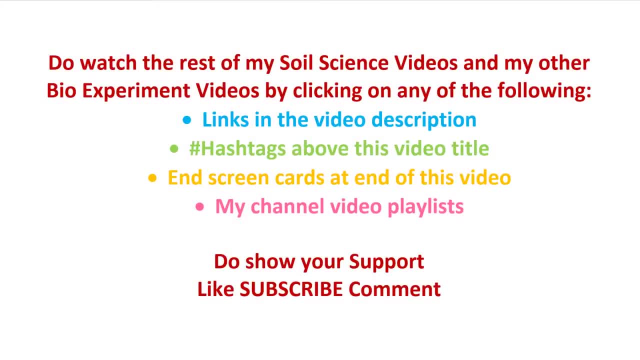 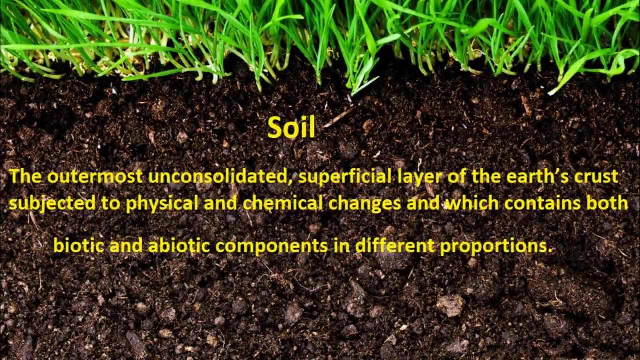 Soil is the outermost unconsolidated superficial layer of the Earth's crust, subjected to physical and chemical changes, and which contains both biotic and abiotic components in different proportions. It is the region on the Earth's surface where geology and biology meet- Soil. 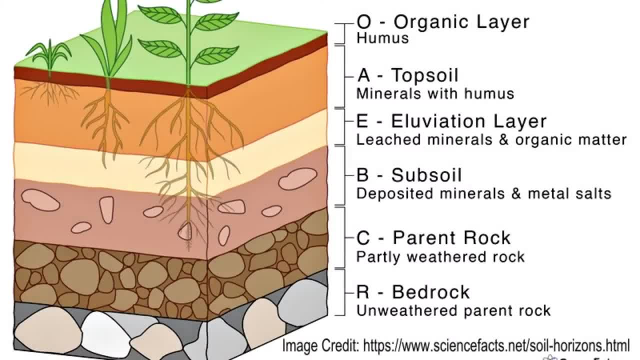 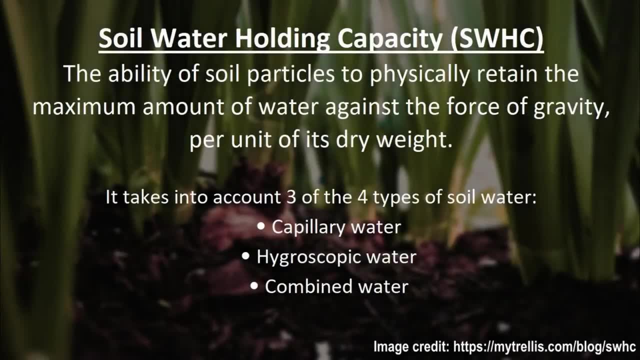 is usually differentiated into horizons of minerals and organic constituents of variable depths. Pseudology is the study of soil. Water holding capacity of soil is the ability of soil particles to physically retain the maximum amount of water against the force of gravity per unit of its dry weight. It takes into account three of the four types. 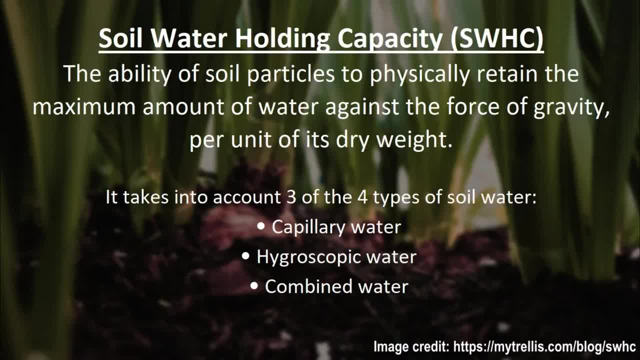 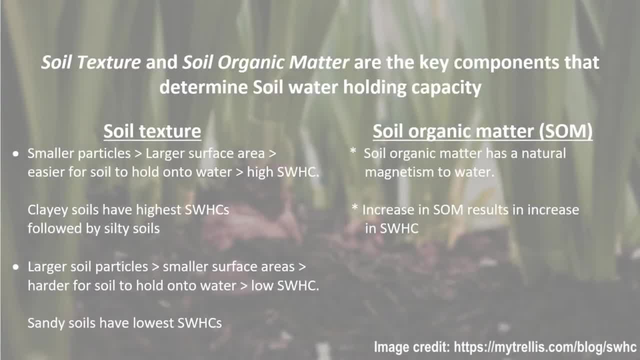 of soil water, that is, capillary water, hygroscopic water and combined water. Soil texture and organic matter are the key components that determine the soil water holding capacity. In terms of soil texture, the smaller the constituent particles, the larger the surface. 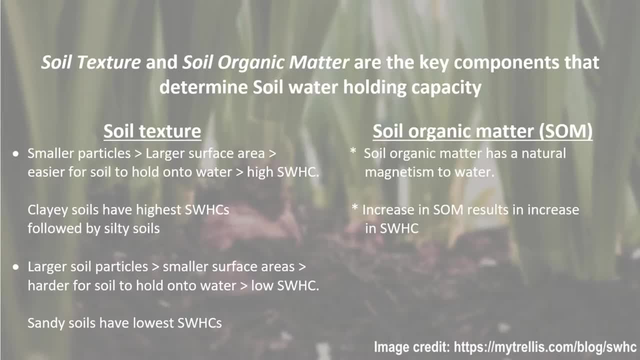 area of those particles and the easier it is for the soil to hold onto water. This results in high water holding capacity. Therefore, clay soils have the highest water holding capacities, followed by silty soils. On the other hand, the larger the soil particles, 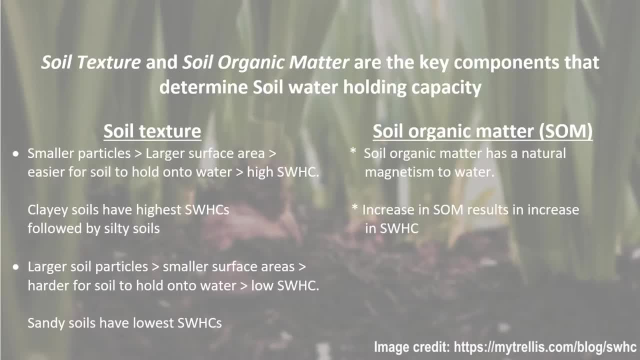 the smaller is their surface area, The harder it is for the soil to hold onto water and, as a result, the lower the water holding capacity. This is why sandy soils have some of the lowest water holding capacities. Each soil texture therefore has its own water holding capacity. 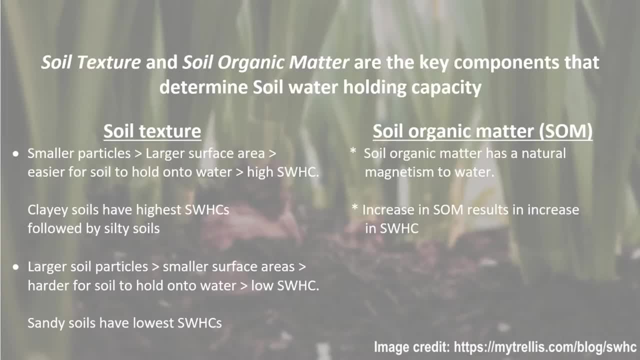 range. Soil organic matter, or SOM, is another factor that can help increase water holding capacity. Soil organic matter has a natural magnetism to water. An increase in the soil organic matter results in a corresponding increase in the soil water holding capacity of the soil. On a more practical note, a good knowledge on the soil water holding capacity 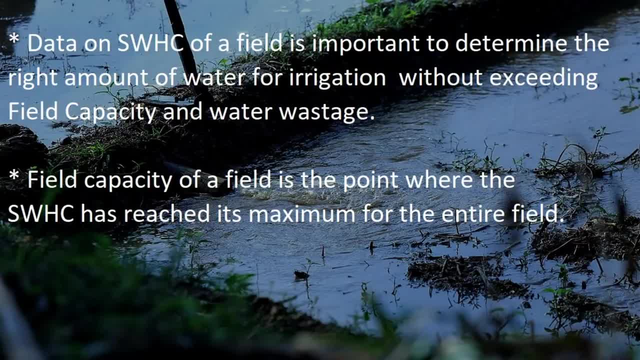 of a field is important to determine exactly how much water needs to be supplied to that field, thus avoiding irrigation beyond the field capacity and eventual water wastage. Field capacity is the point where the soil water holding capacity is the point where the soil water holding capacity has reached its maximum for the entire field. In this, 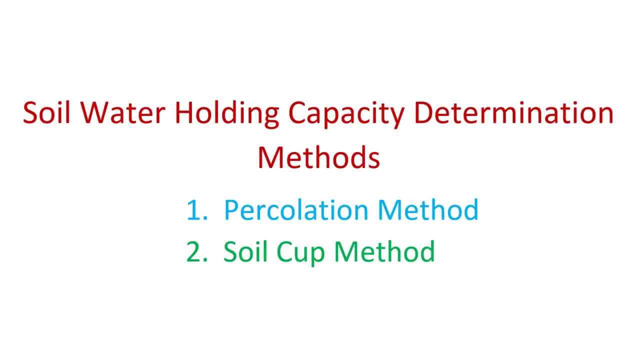 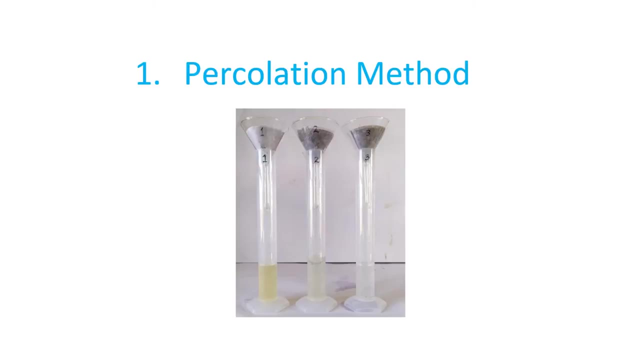 experiment video. we'll be discussing two methods to determine the water holding capacities of three different soil samples collected from three different locations: the percolation method and the soil cup method. The following materials are required to perform the test using the percolation method: Three soil samples that were oven-dried for 24 hours and finely. 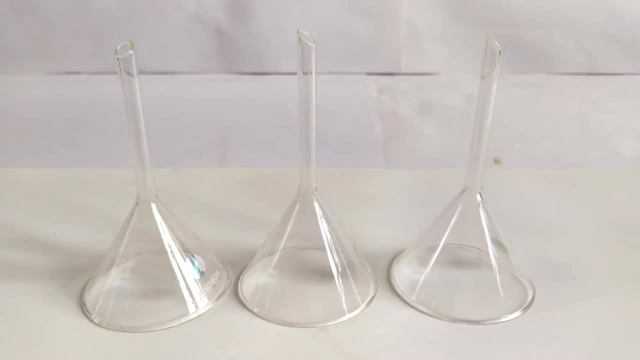 powdered prior to the start of the soil water holding process. The soil water holding capacity of the soil water holding capacity is the point where the soil water holding capacity is the start of the soil water holding process. The soil water holding capacity is the point where the soil water holding capacity begins. The soil water holding capacity is the point. 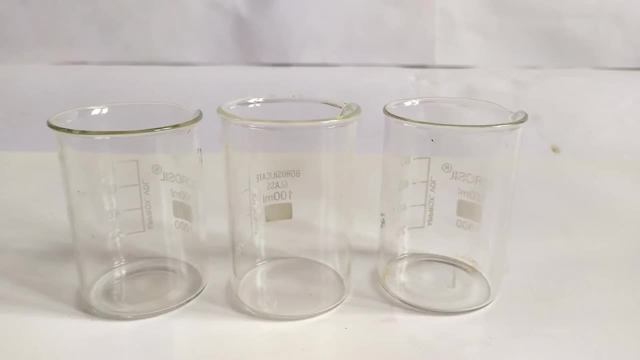 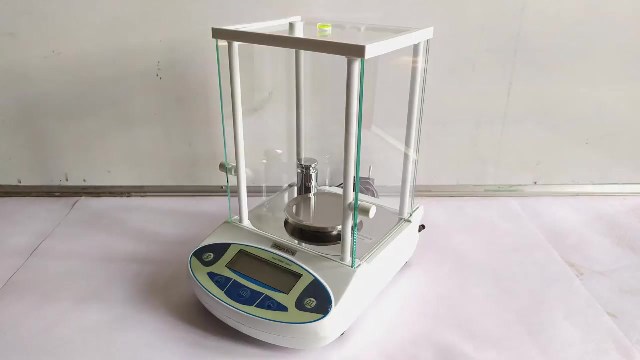 where the soil water holding capacity begins, followed by the super must, an mathematical beberace brings in the soil water hanging capacity. For soil water holding capacity, thesigh should crust or solid就是說 the soil water holding capacity Instysttion. 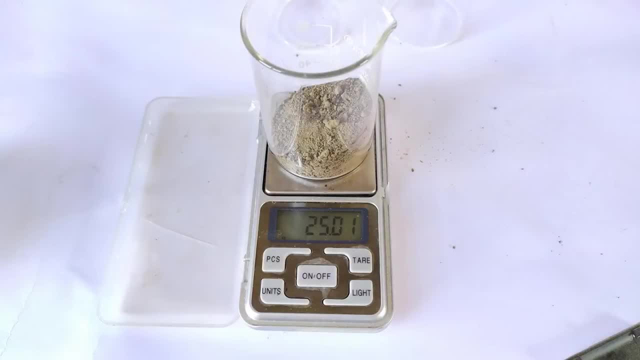 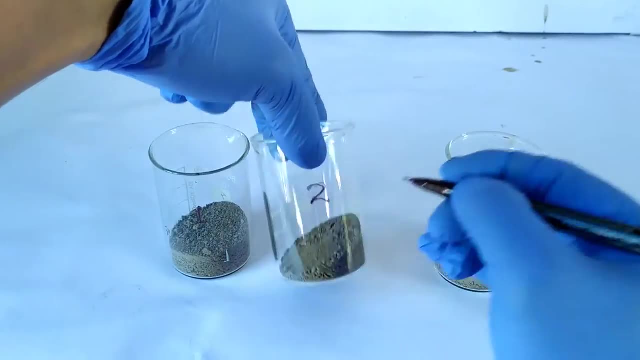 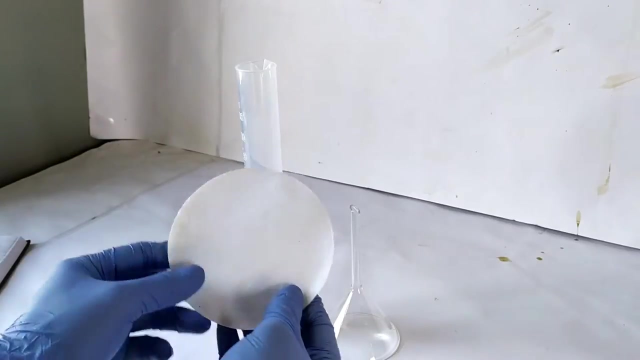 Take three soil samples and weigh about 25grs of each sample. at the beginning of the experiment, Label the containers inside and keep them in one place and proceed to prepare the percolation percolation setups. To make this setup, take a filter paper circle, fold it twice as seen here and open one of 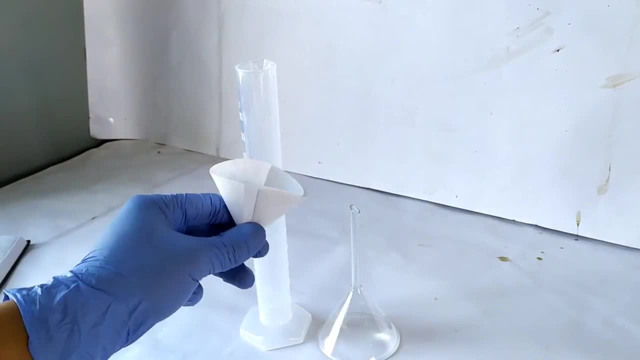 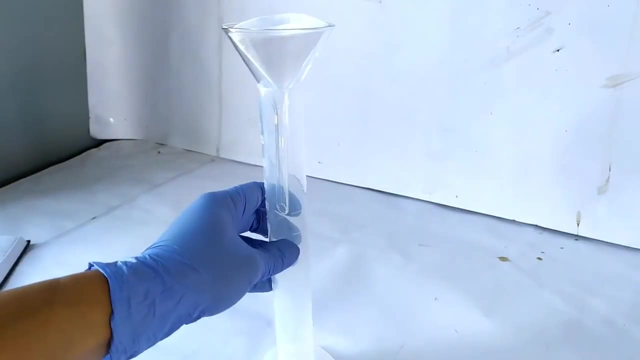 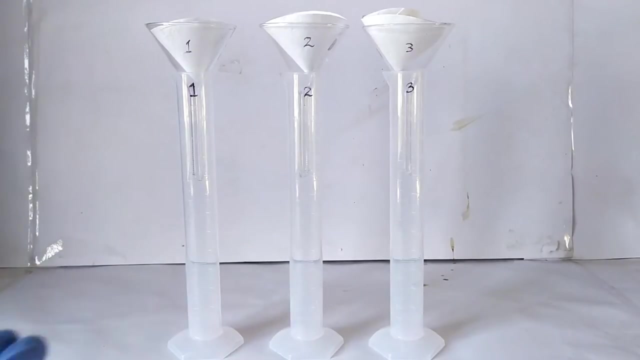 the folds to make a cone like this. Insert this filter paper cone into a funnel like so. Place this funnel in the mouth of a graduated cylinder. This is the percolation setup. Prepare three such identical, appropriately labeled setups for all the three samples of. 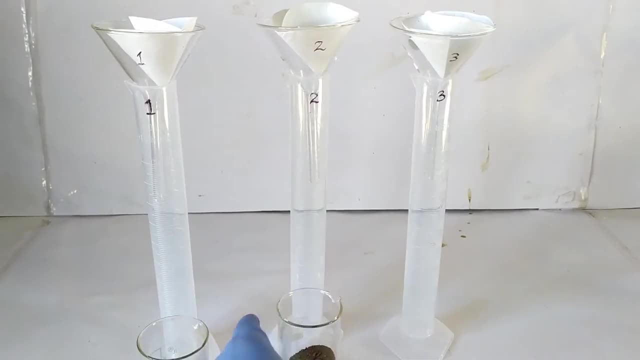 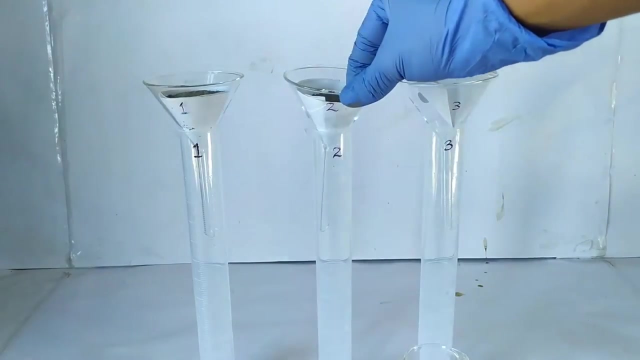 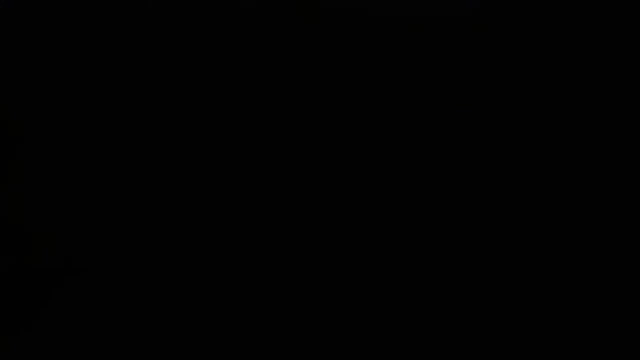 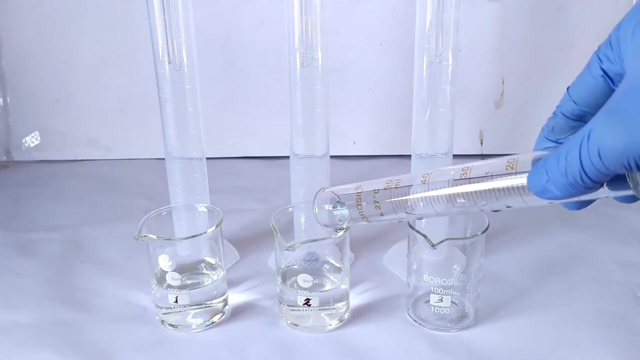 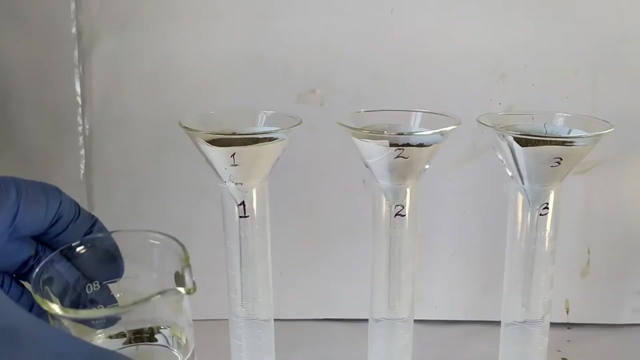 soil. Now take the three pre-weighed soil samples and carefully pour them one by one into the filter paper cones of the three funnels. Now introduce 50 ml each of water into three labeled beakers. Carefully add the water from each beaker into the three soil-containing funnels in small 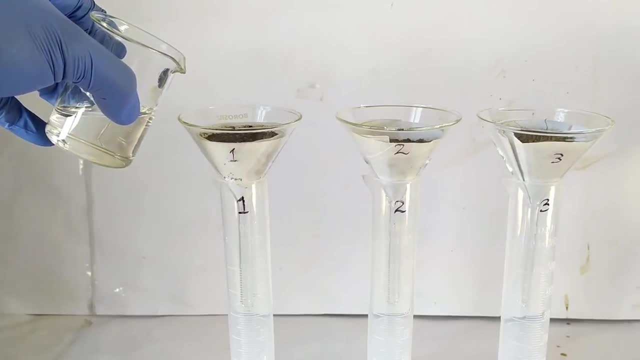 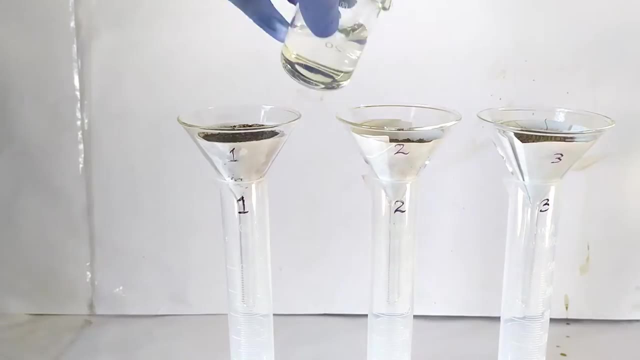 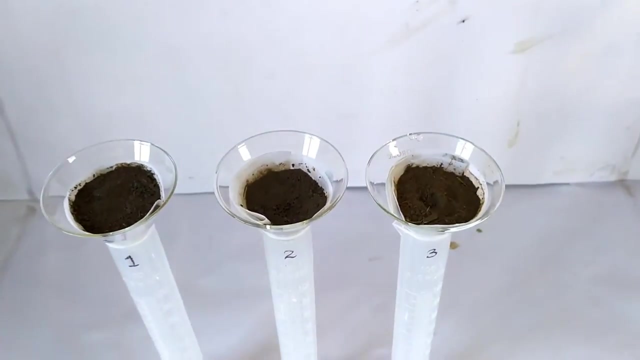 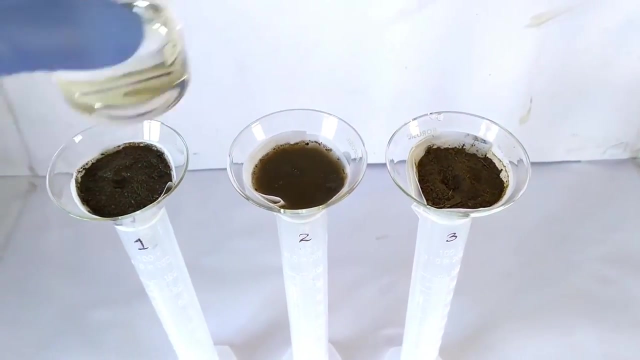 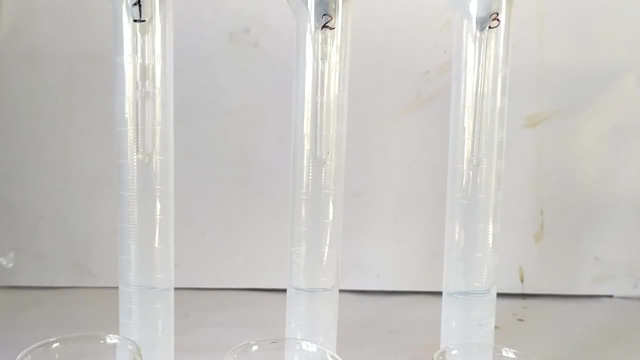 increments. Do not add water beyond the level of the filter paper cones. As you keep on adding water, it will eventually seep through the soil, samples trickle down through the funnels and get collected in the graduated cylinders. Once all the water contents of the beakers have been poured into the funnel, leave the 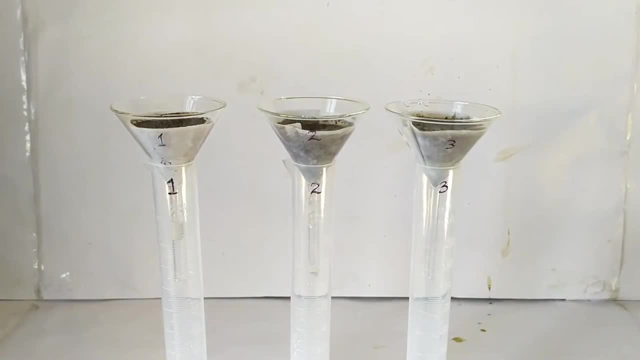 percolation setups undisturbed for several minutes until no more water trickles through the stem of the funnel and the soil samples are ready to be poured into the funnel. This is the final step. Now the soil samples get completely saturated with water. 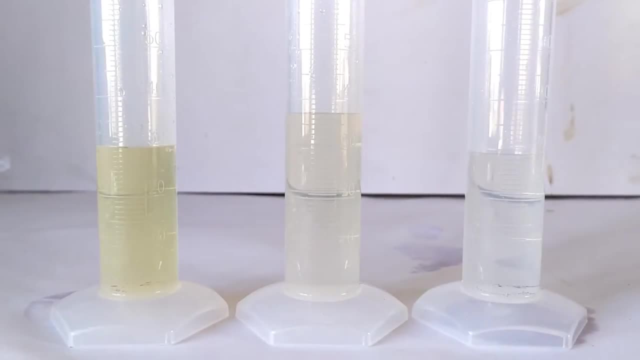 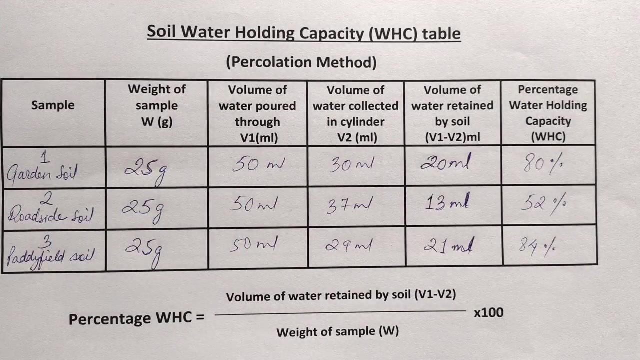 Now measure the volume of water collected in each of the three cylinders. Table 8: your observations, as seen here, Do the math and determine the water holding capacity of each soil sample in terms of percentage. We can see from this experiment on three soil samples that sample 1 has a water holding. 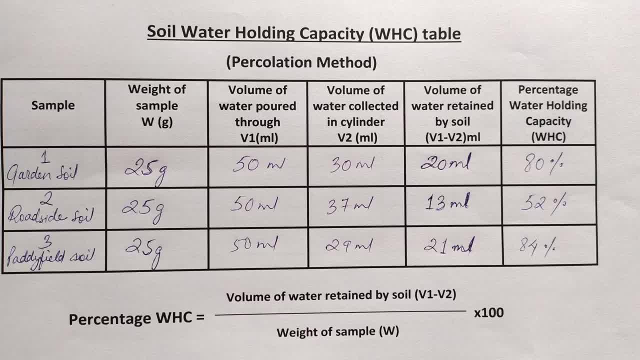 capacity of 80%, sample 2: 52% and sample 3: 84%. Now let's see the results. We can conclude that soil sample 3,, which is a paddy field soil sample, has a maximum water holding capacity of more than 80% and can therefore be considered to have more of. 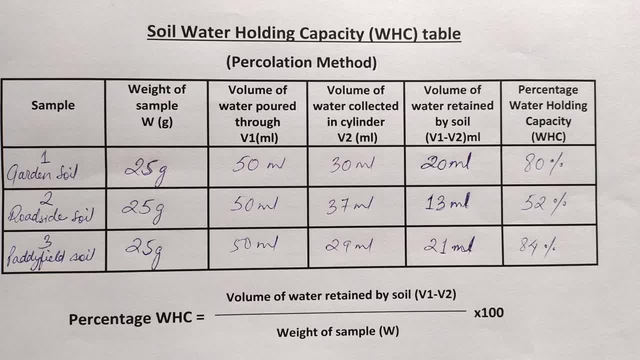 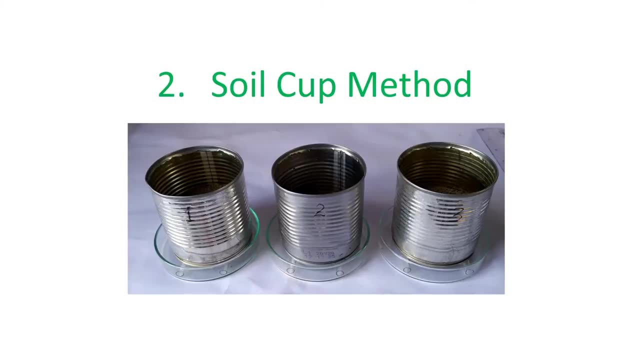 a clayey character. Sample 2,, on the other hand, has the least capacity of a little over 50% and can be considered to have more of a sandy characteristic compared to the other two samples. To perform this method for three samples of soil, the following materials are required: 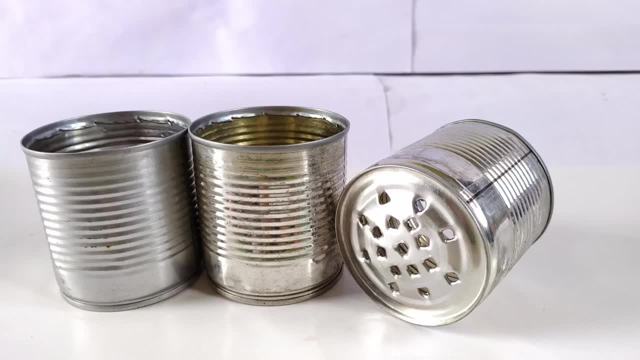 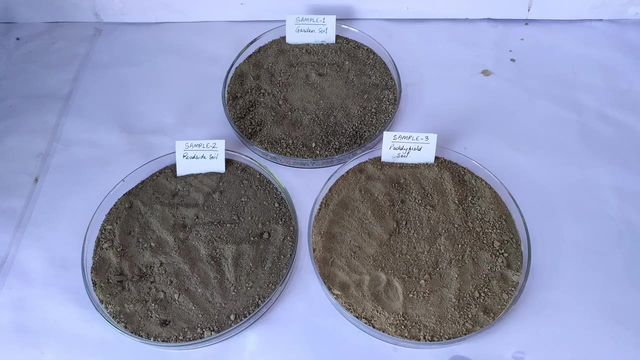 The following materials will be required: Three soil cups with perforations at their bottom- You can easily make them from three identical tin cans by making perforations at the bottom of the cans using a nail and hammer or such similar device for punching holes. Three soil samples that have been oven dried overnight and ground into a powder prior to. 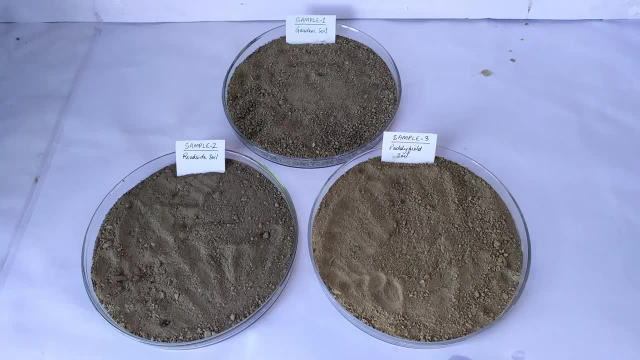 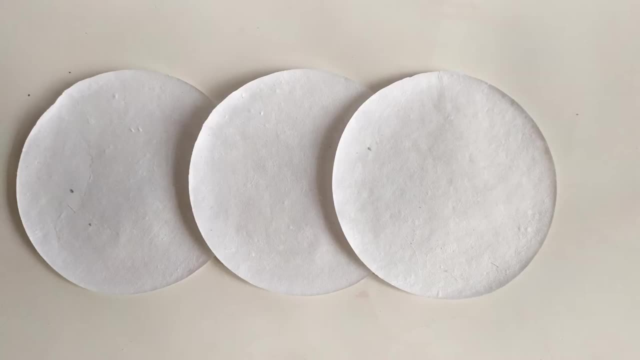 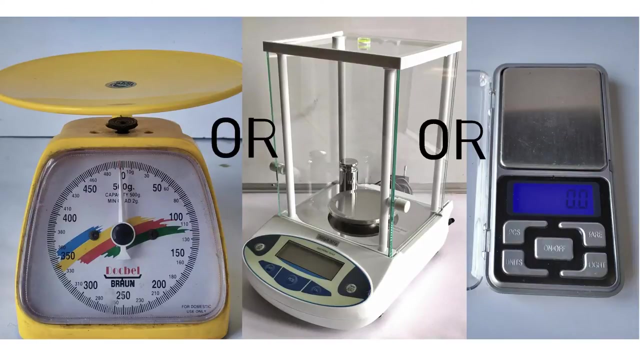 the start of the experiment. For convenience, we take the same set of samples used in the previously discussed percolation method: Three identical petri dishes or beakers, Three filter paper circles, Three pairs of short glass tubes Weighing scale. 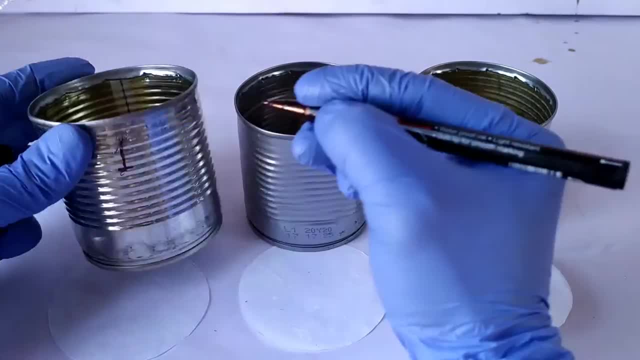 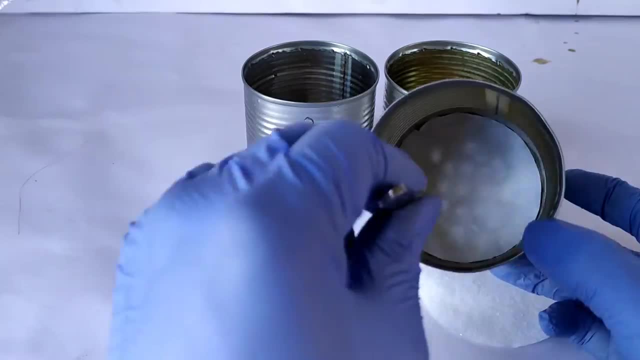 To begin, take the three soil cups and label them appropriately. At the perforated bottom of each of the soil cups insert a sheet of filter paper each that have been pre-cut to perfectly fit the bottom of each of the soil cups. The soil cups can beoperated to the soil easily. 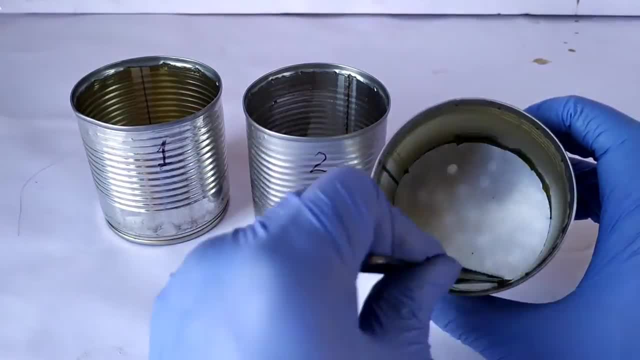 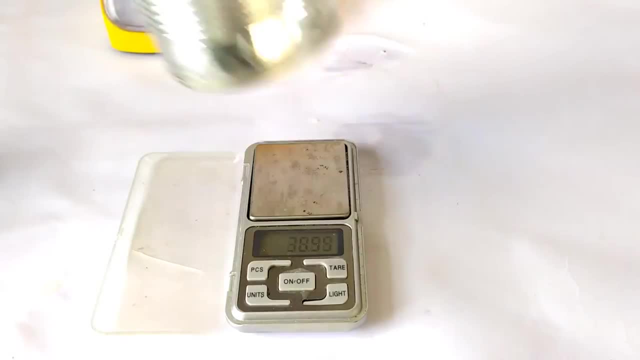 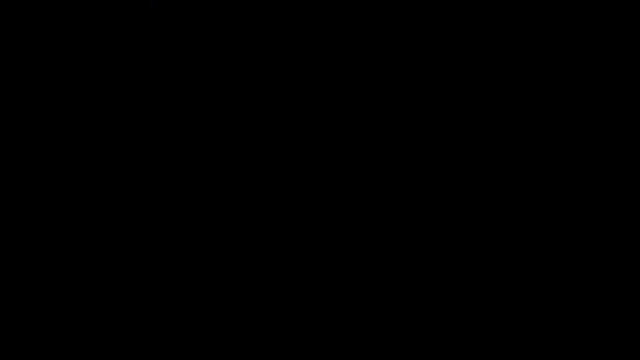 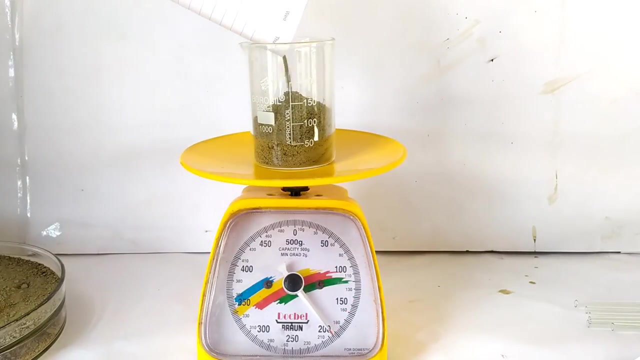 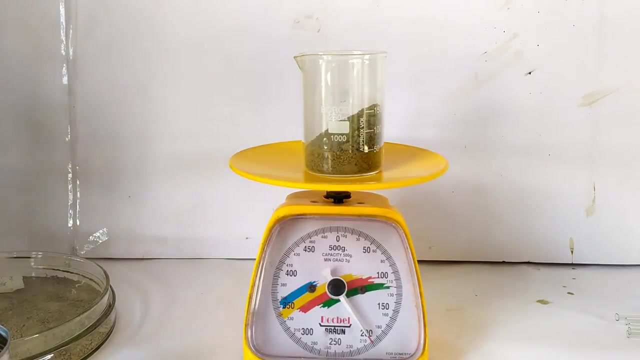 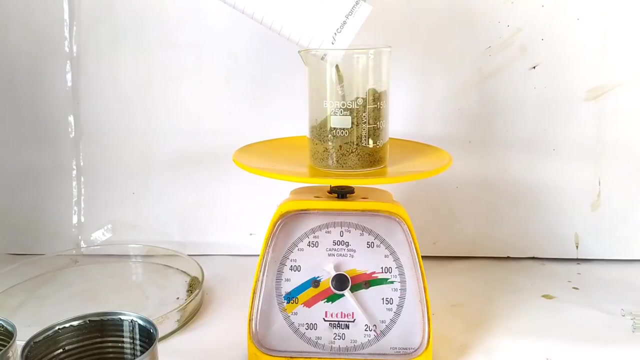 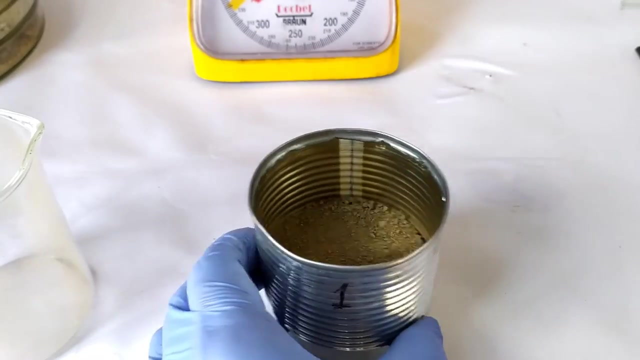 cup as seen here. Now weigh the empty cups one by one and record the weights. Also, weigh 100 grams each of the three oven-dried soil samples. Introduce each sample into the corresponding pre-labeled empty soil cup. Gently agitate and tap the cups to allow a uniform. 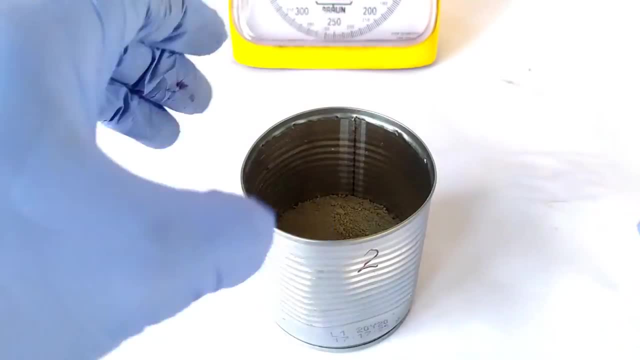 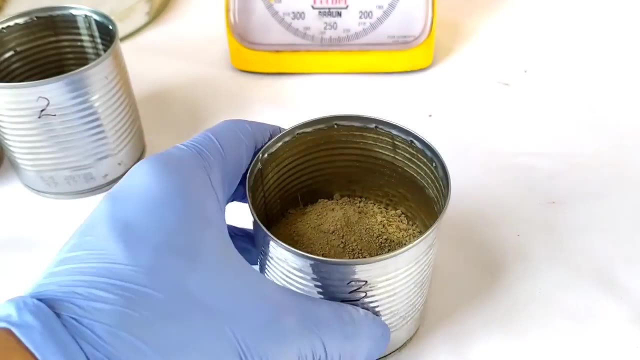 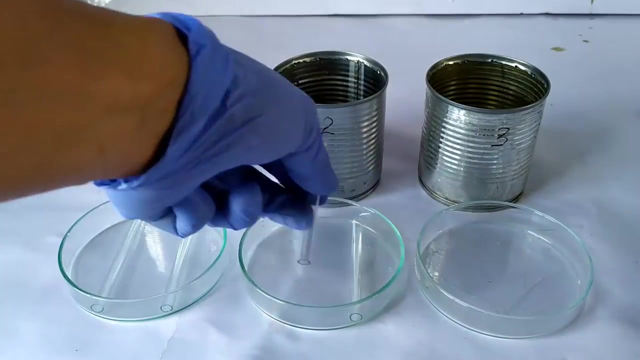 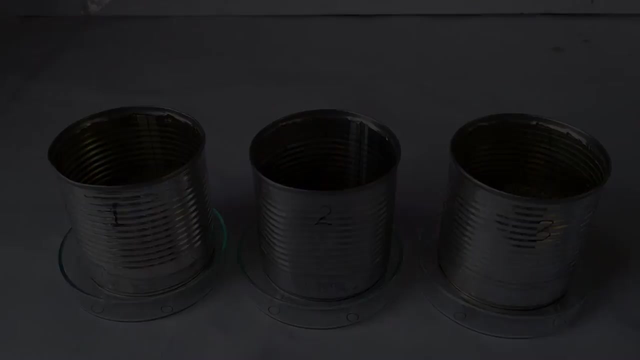 difference. Now. place two short glass tubes, at a distance from each other, into each of the three beakers or petri dishes. Place the soil cups on top of the glass tubes in the beaker or petri dish, like so. Carefully introduce some amount of water into the petri dishes, such that 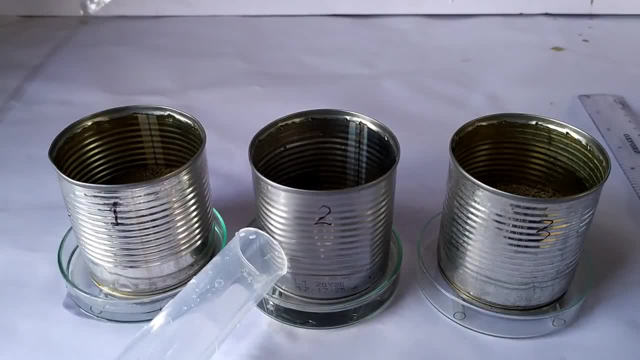 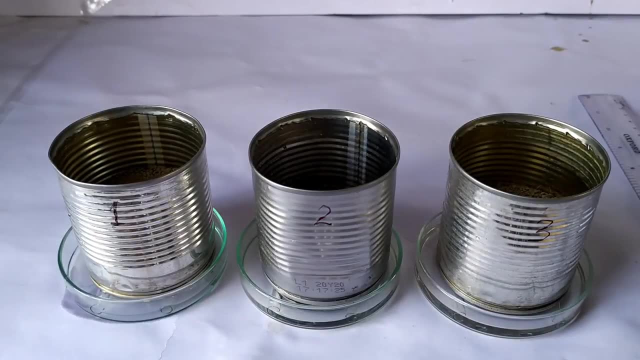 at least the bottom 1 cm of each of the soil cups is immersed in the water. Leave the three setups undisturbed for some time and observe the surface of the soil samples at every interval. You also might have to constantly refill the water in the petri dishes as the soil samples. 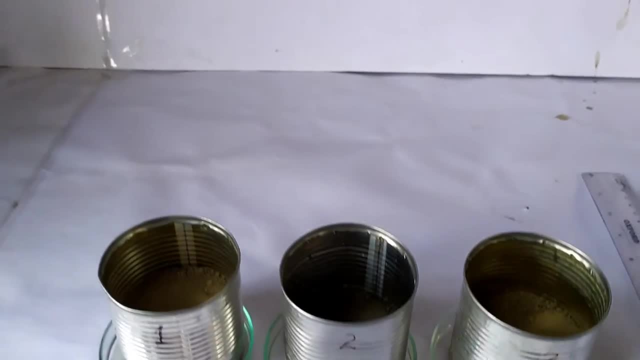 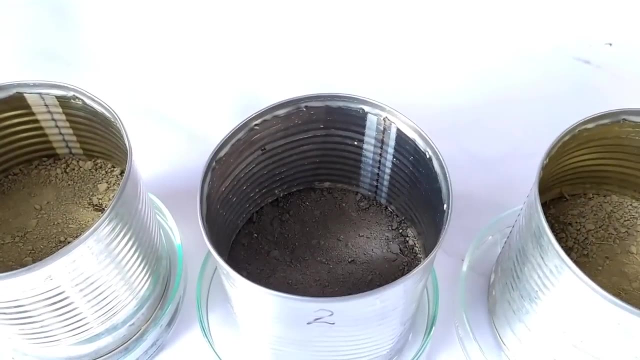 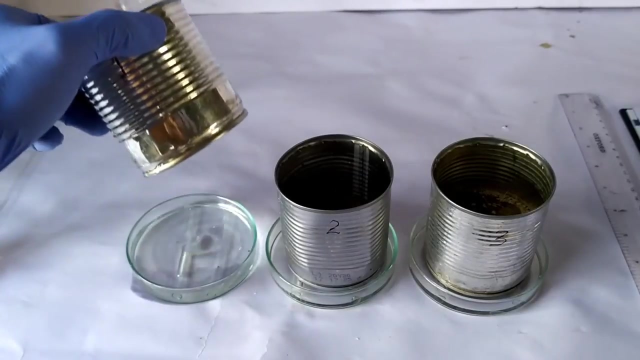 continue to absorb the water. Once the level of the water reaches the soil surface, such that the soil becomes thoroughly soaked in water, but not so much as to cause water logging, as can be seen in one of the samples here, Remove the soil cups carefully from the petri dishes. hold the cup elevated for a few minutes. 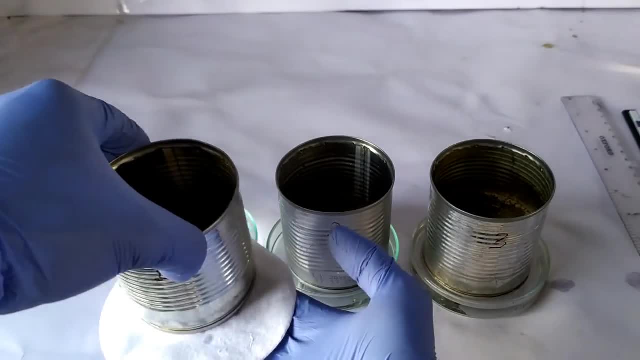 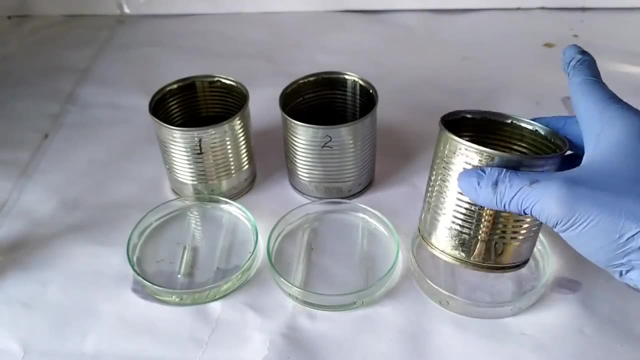 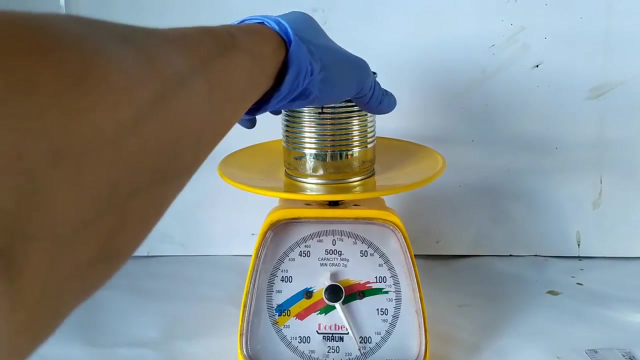 and dab the bottom of the cup using blotting papers until no more water drops trickle from the bottom of the soil cups. Once excess water has completely drained, weigh the soil cups again and record their weights. You can see that the soil cups are now completely soaked in the water and the soil samples are.